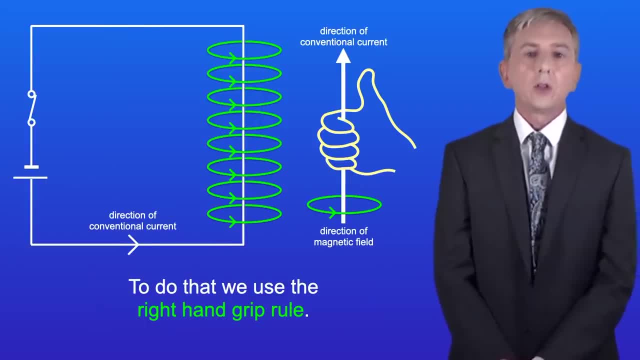 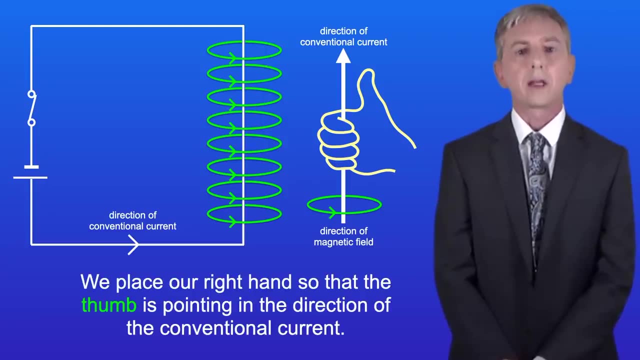 the direction of the magnetic field produced by a wire. To do that we use the right-hand grip rule and I'm showing you that here We place our right hand so that the thumb is pointing in the direction of the conventional current. Now the fingers are pointing in the direction of the magnetic field. 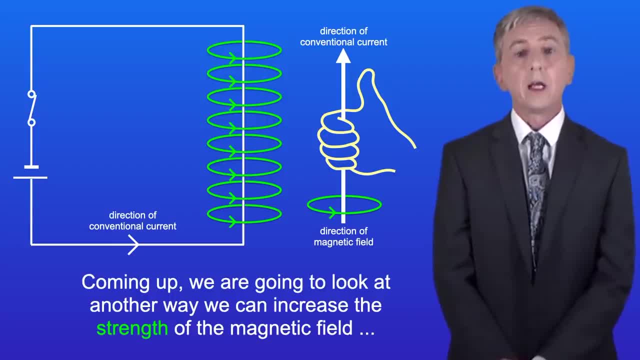 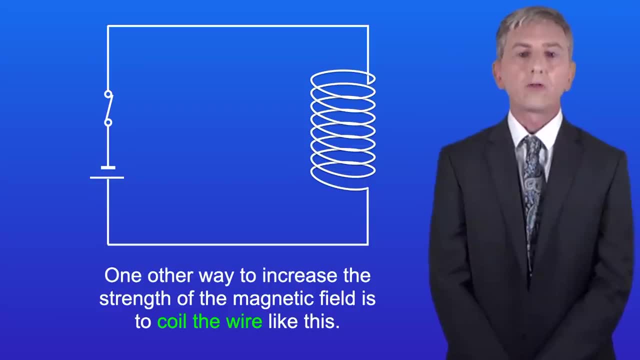 Coming up. we're going to look at another way we can increase the strength of the magnetic field in a wire carrying an electric current. OK, now, one other way to increase the strength of the magnetic field is to coil the wire like this. Scientists call this shape a solenoid, and 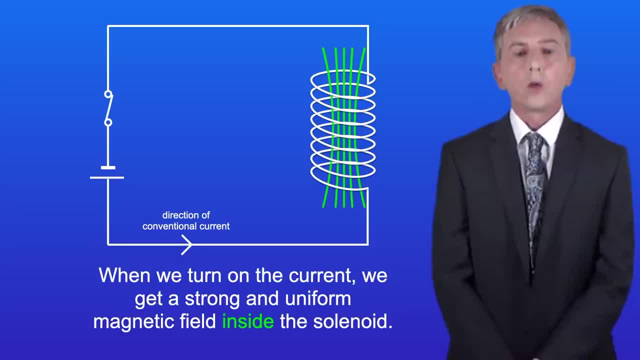 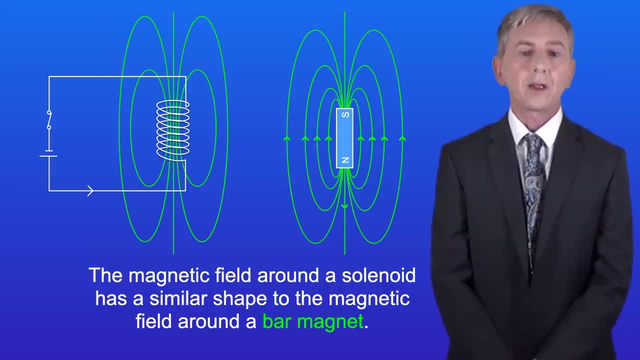 you do need to learn that name. When we turn on the current, we get a strong and uniform magnetic field inside the solenoid. The magnetic field around a solenoid has a similar shape to the magnetic field around a bar magnet and I'm showing you that here Again in the exam you could be asked to. 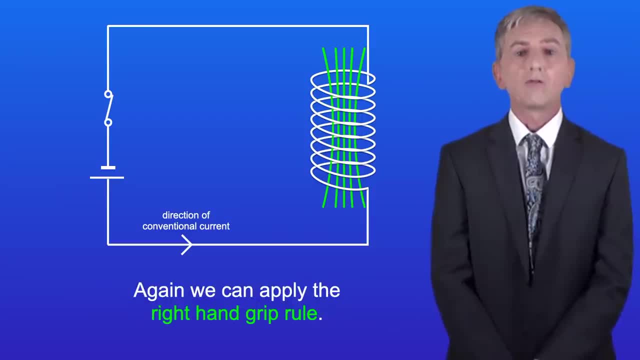 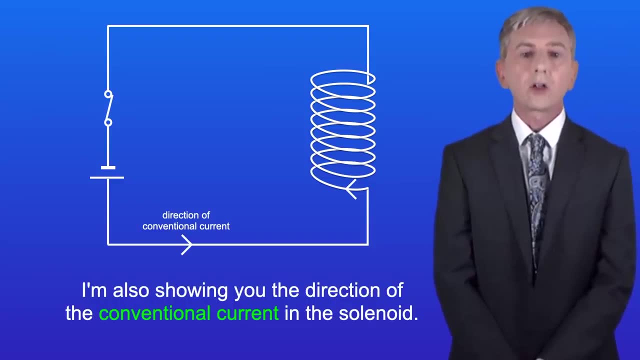 work out the direction of the magnetic field and again we can apply the right hand grip rule. To make this easier, we're going to remove the magnetic field lines. I'm also showing you the direction of the conventional current in the solenoid. In this case, place the fist of your right hand so the fingers curl in the 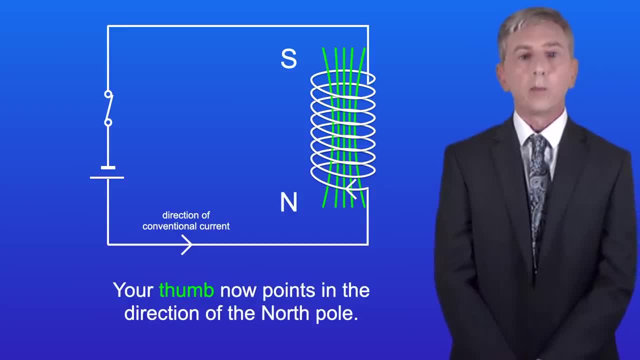 same direction as the solenoid. Now we can see that the magnetic field is in the same direction as the conventional current. Your thumb now points in the direction of the north pole. Now there are three ways we can increase the strength in the magnetic field. 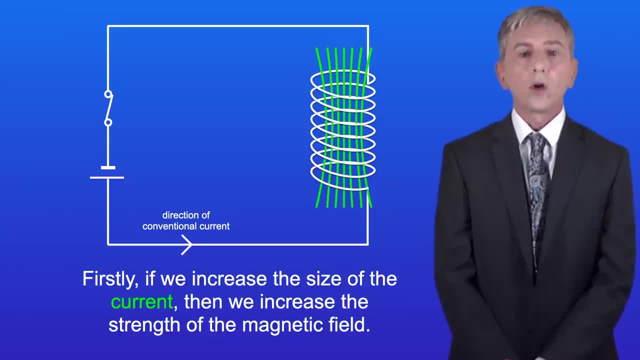 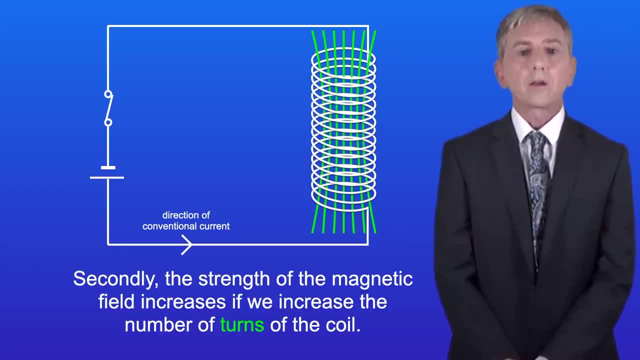 produced by a solenoid and you need to learn these. Firstly, if we increase the size of the current, then we increase the strength of the magnetic field. Secondly, the strength of the magnetic field increases if we increase the number of turns of the coil. 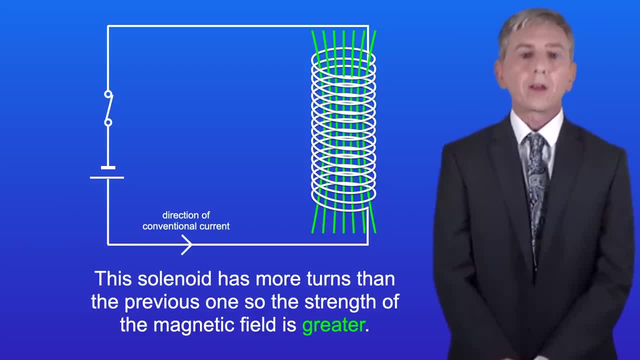 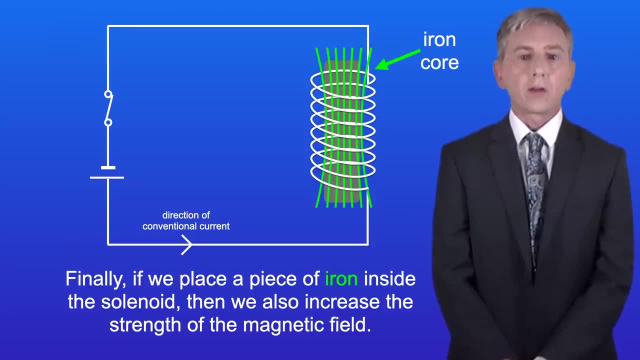 This solenoid has more turns than the previous one, so the strength of the magnetic field is greater. And finally, if we place a piece of iron inside the solenoid, then we also increase the strength of the magnetic field. Scientists call this an iron core, Now a solenoid containing an iron core. 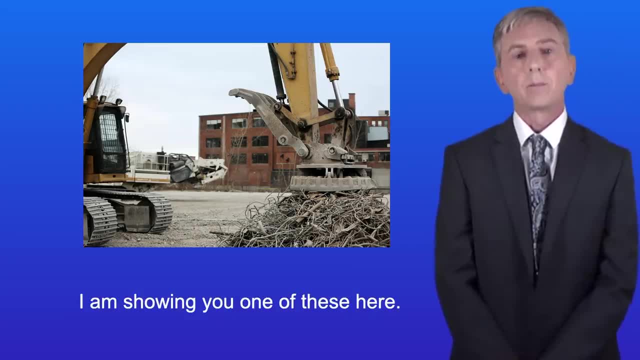 is called an electromagnet, and I'm showing you one of these here. Electromagnets are extremely useful, as we can change the strength of the magnetic field by changing the size of the current. We can also turn an electromagnet on or off.